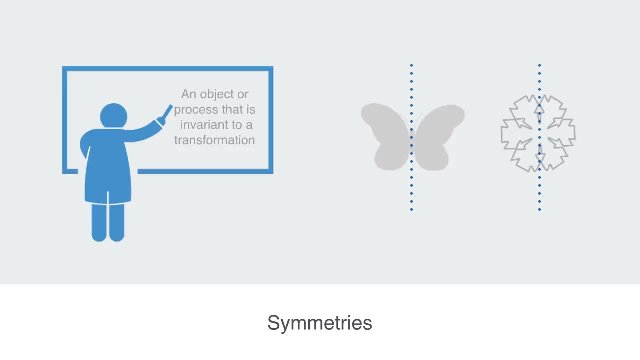 So with our example of the butterfly, its external physiology had a relationship with the earth, Meaning we can simply flip one side over and we'll get the other side. The same was true of our snowflake, and we can imagine some symmetry in the pattern of earth's orbit. 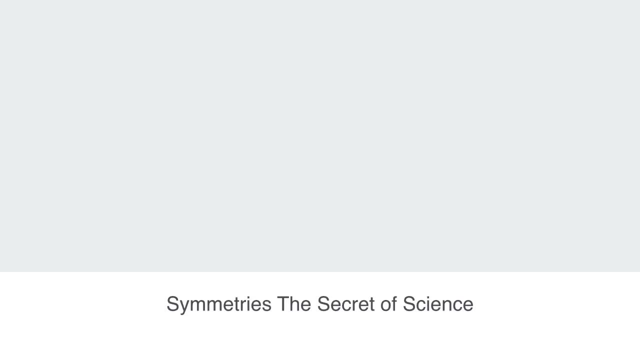 Without these symmetries to our world, the scientific endeavour would be very difficult, because science is about the creation of compact representations of the world. It is like we're creating a map of the world, and it is only through finding these symmetries and encoding. 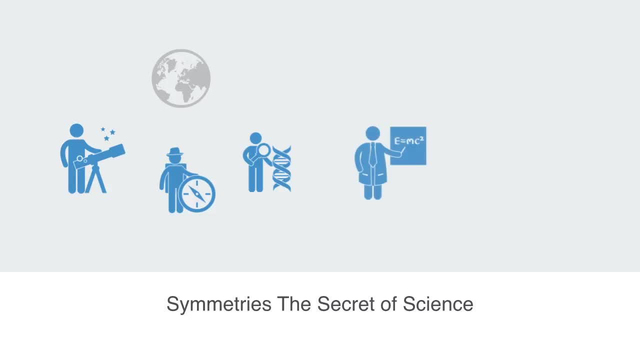 them in models that we can describe a wide variety of phenomena with simple equations. Without these symmetries, our scientific map of the world would have to be the same size as the world itself, and thus useless. Symmetry and its counterpart, asymmetry, are, then, two of the most powerful concepts in mathematics and science. 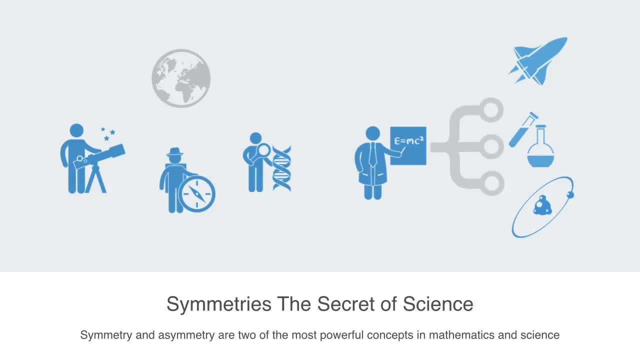 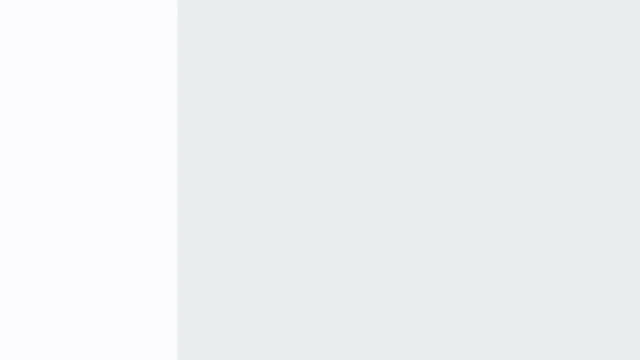 For talking about order and chaos. they help us to understand these abstract concepts in a distinctly geometric and visual form. So with the phenomena of chaos, we saw this breaking of symmetry, as two things that started out similar became increasingly dissimilar as the symmetry between them became broken and the result was, after a short period of time, complete asymmetry. 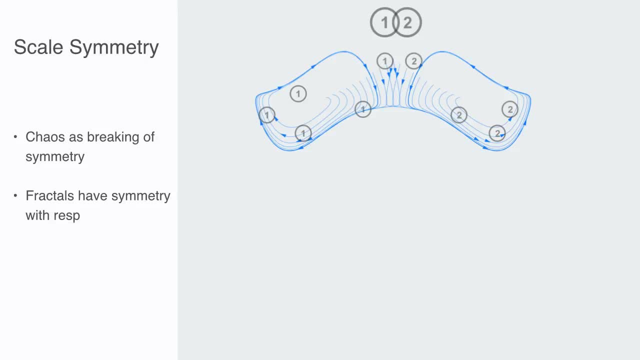 Fractals have what is called scale invariance, that is, they have a symmetry with respect to scale, meaning the scale can change, but the structure will repeat itself over various levels of magnitude. This scale invariance is also called symmetry. 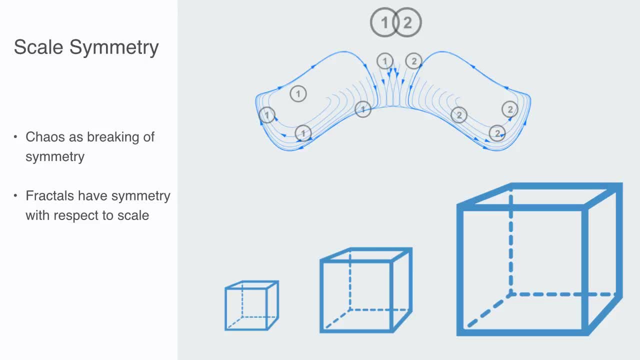 This is called self-similarity, and it is this type of symmetry under magnification that defines fractals and gives them an amazing type of structure and order. Fractals are both mathematical constructs that derive out of iterative functions and real-world phenomena. 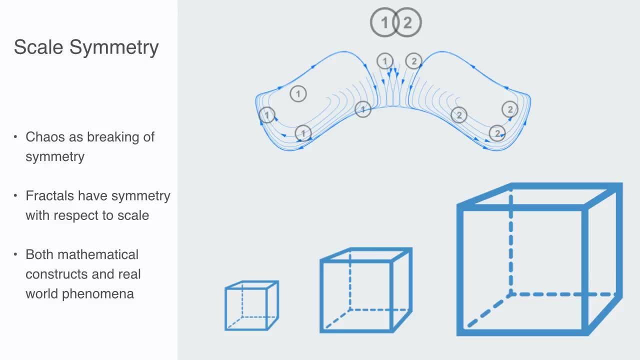 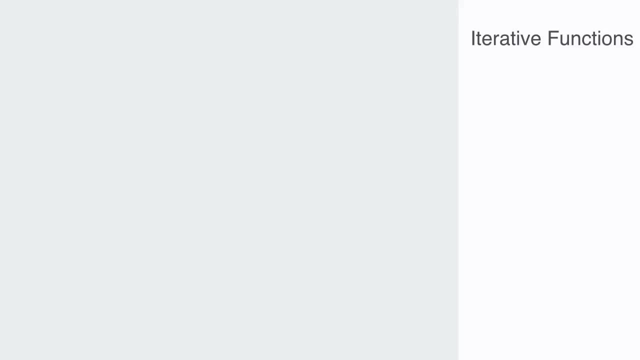 In this module we will present them as mathematical models and then in the next, look at their real-world counterparts. As we have seen with most of non-linear systems, the core ideas behind fractals is a feedback and iteration. The creation of most fractals involves applying some simple rule to a set of geometric forms or numbers. 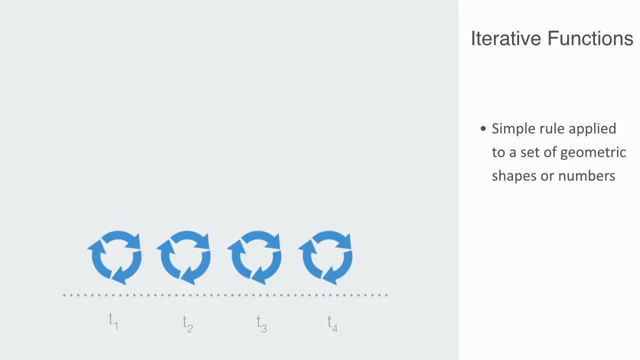 and then repeating the process on the result. For example, the most famous fractal, called the Mendelbrot, set so named after the discoverer of the concept of fractals, is a product of a simple iterative function on complex numbers. 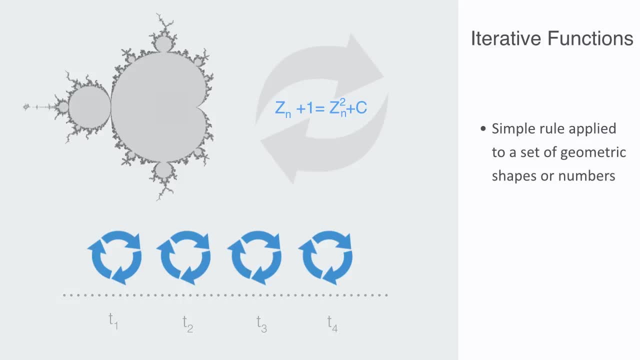 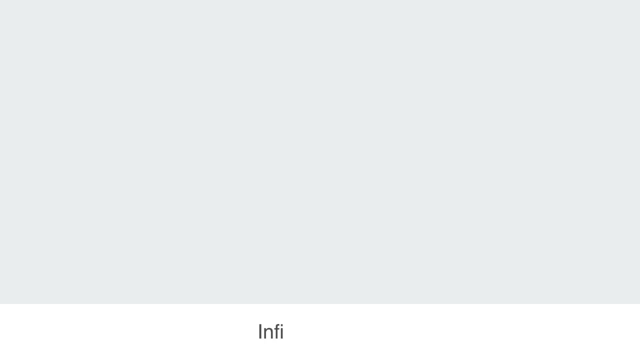 We will not go into the details of complex numbers, but the iterative math itself is quite simple. There are many extraordinary things about fractals, but the first thing we will note is the infinite variety that these simple iterative functions can produce, Whereas most Euclidean shapes- what we might call normal shapes- tend towards a bland featurelessness as we scale them up. 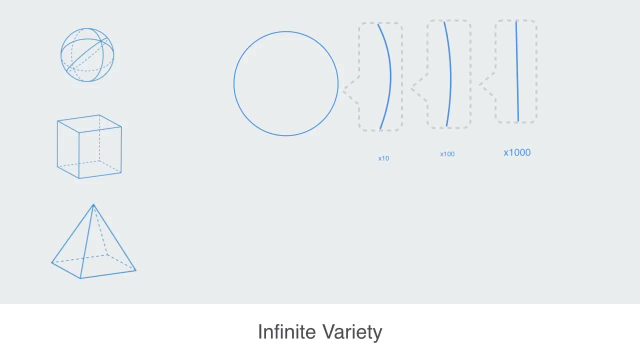 If we take something like a circle, the more we zoom in on it, the more it will start to appear like a bland straight line, and this would also be the case for other regular shapes such as squares, triangles and so on. The iterative functions behind fractals. in contrast, 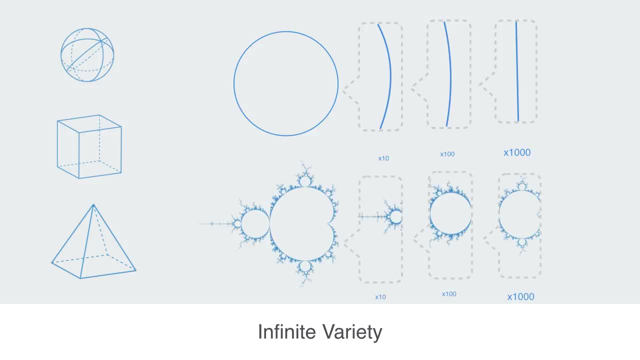 give us an infinite amount of detail and structure within their form. Irrespective of if we divide the shape into two or divide it into a million, each of these million little parts will itself have an infinite amount of detail and a form that resembles the whole. 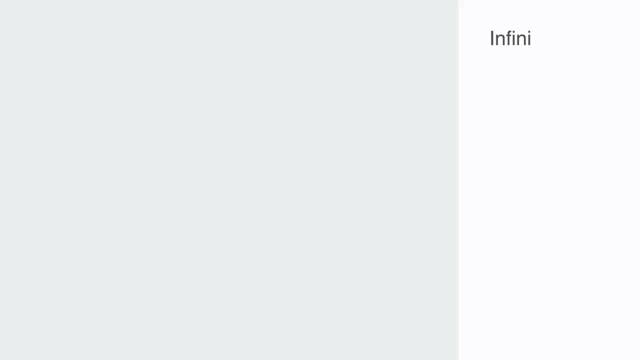 Just as there can exist an infinite amount of form in a finite object, there can, in fractals, also exist an infinite length within a finite length. This is best demonstrated by a fractal called the Koch curve That can be obtained by iterating a simple process of dividing a line and placing a triangle in its centre. 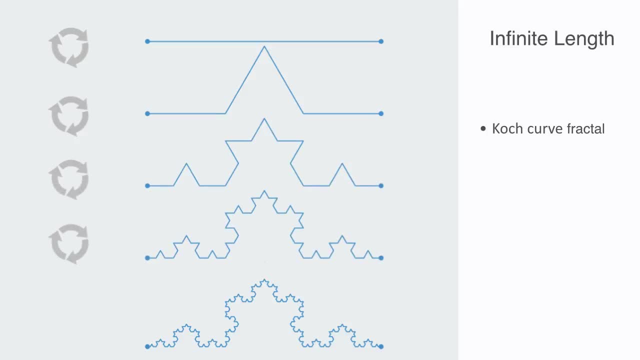 and then, iterating on this, to divide the line on the triangle in a similar fashion. What we get when we do this is a path that will, in fact, have infinite length to it. If we were to try and trace a path along this line, its infinite detail would prevent us from ever reaching the end. 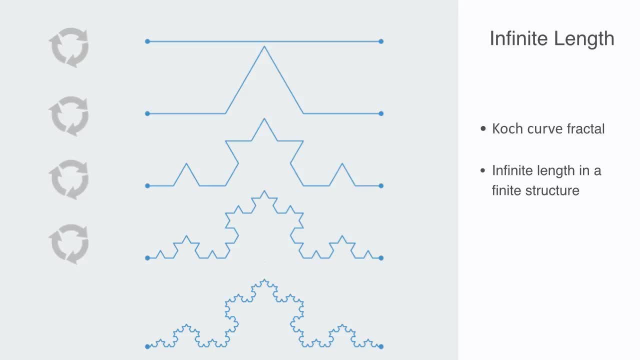 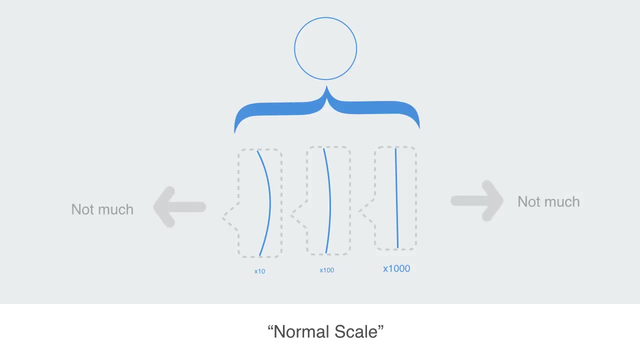 Thus, this finite length contains an infinite length within it. The last thing we'll note about fractals is their scale-free property, meaning that no scale is the proper frame of reference. Most linear systems that represent regular forms have features and structures within a limited range of scales. 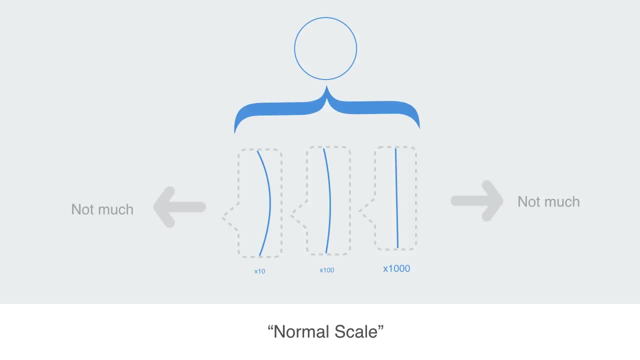 Thus, if we plot these features, we would get a normal distribution with the majority of features tending towards some kind of mean, giving it some kind of normal frame of reference. with respect to scale, These non-linear fractals, as we've noted, have scale invariance.